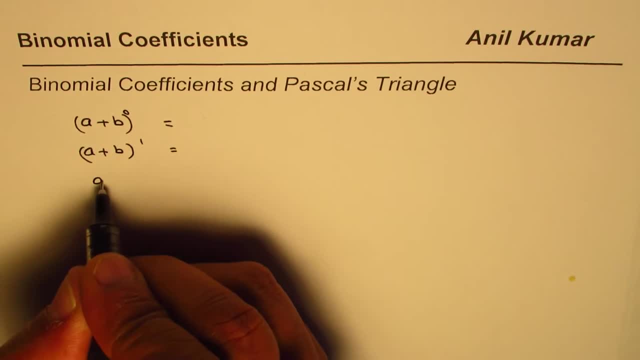 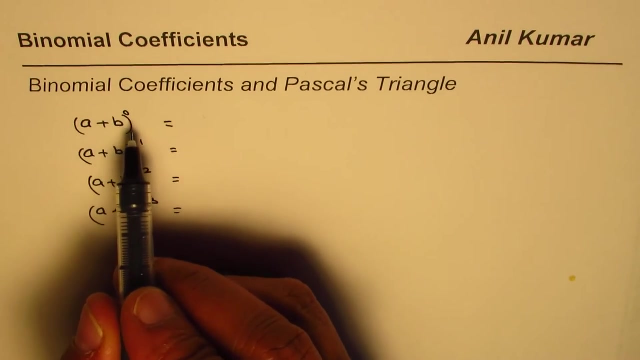 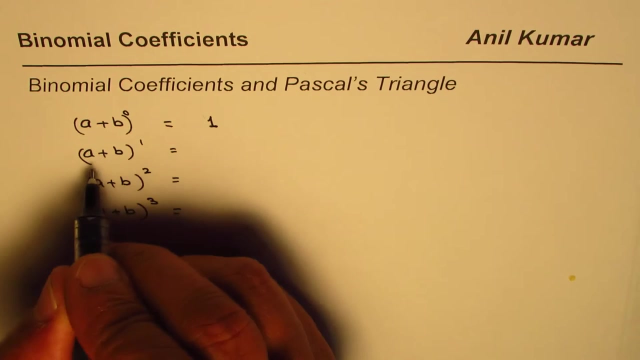 and if you expand it, what do you get? if I have a plus b whole square, then what is the result? and if you have a plus b whole cube, then what do you get? Now? anything to the power of zero, as you know, is one. anything to the power of one is the number itself, which, in our case, is the binomial. 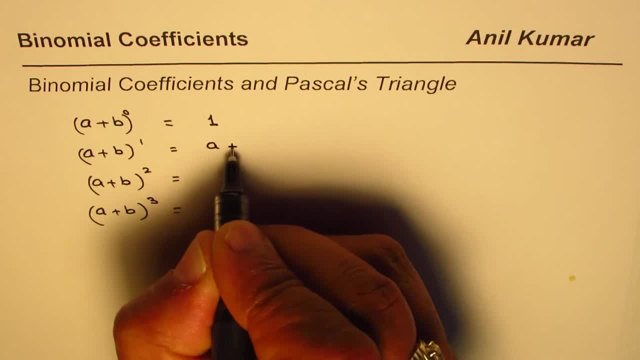 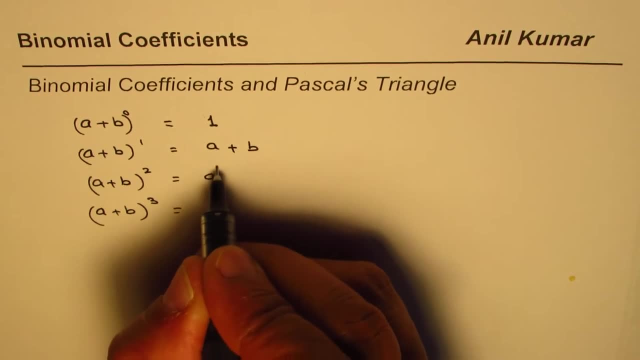 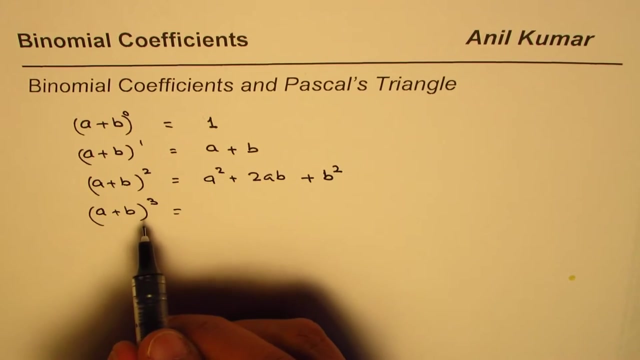 a plus b. So we get a plus b right. but if case we have a square, then we know the formula. it should be a square plus two, a, b plus b square. For q we can multiply a square plus two, a, b plus b square by a plus b. 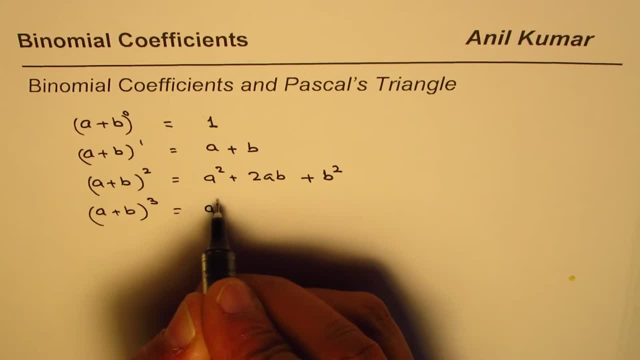 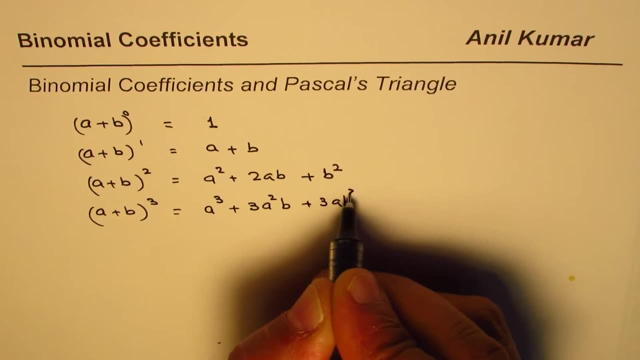 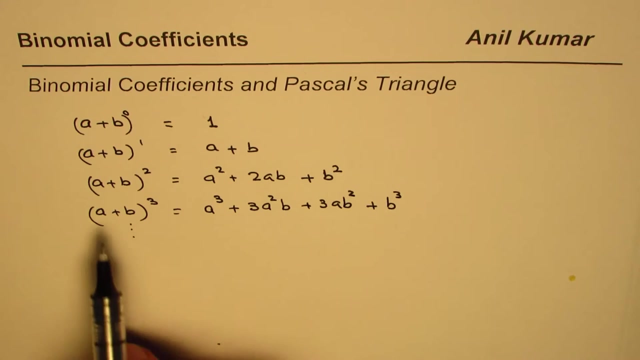 expand and simplify, then what we get here is a cube plus three a square b plus three a b square plus b cube, right? Similarly we can continue. So once we expand and simplify, we'll get few terms, as shown here. Now, important thing here is that when this exponent, let's say: 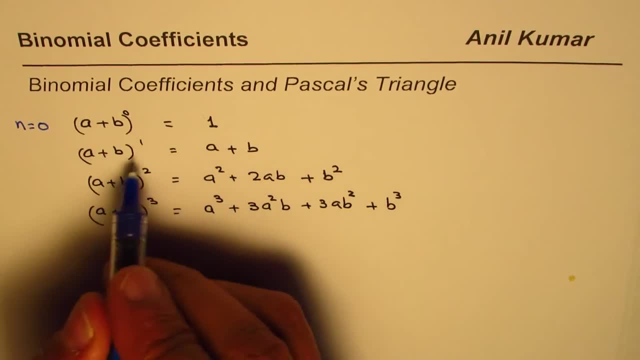 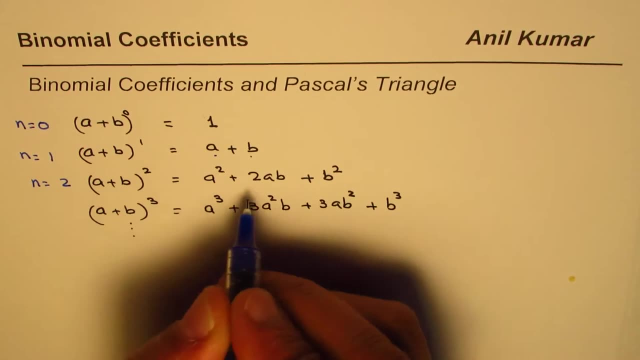 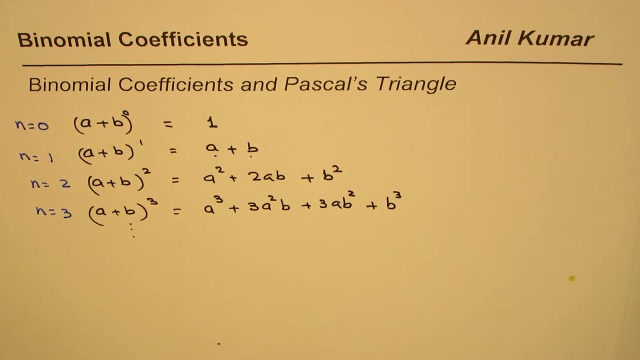 the exponent n is zero, we get one term. when the exponent n is one, we get two terms. when the exponent is two, we are getting three terms. So we get two terms. when the exponent is one, we get two terms. When the exponent is three, we get aола. we get three terms. So number of 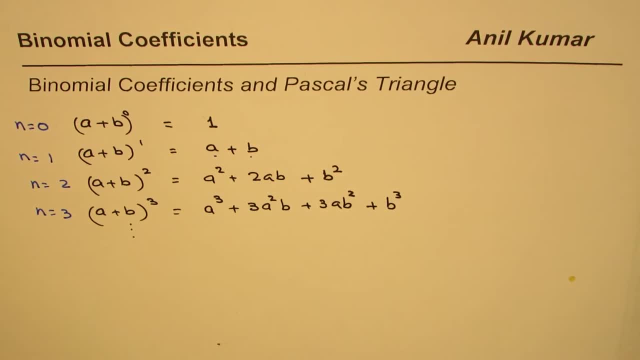 three terms. when the exponent is three, we get four terms. so number of terms is one more than the exponent. that is what we see. We also observe that the exponents are same as n. here we could say that the power of zero and b to the power of zero. 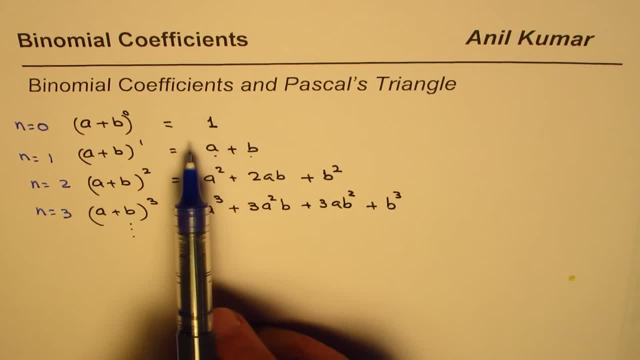 or one create. so anything to the part, use one: 1. 1.. So therefore we have: we get four terms together: 1. 1.. here we could choose a to the power of zero. that means the exponents when they get added up, it's kind of same as n, right here? a when you write a, 1 is the. 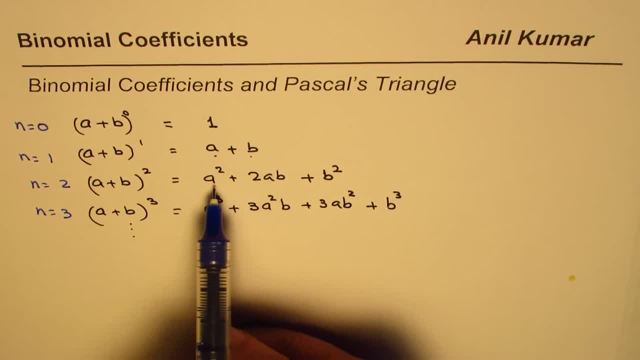 exponent for B. 1 is the exponent, so the exponents are 1. in this case it is more clear. a square. the exponent is 2, same as that here. what is the degree of this term, the term to a, B? when you combine 1 and 1, 1 plus 1 is 2. again the degree is: 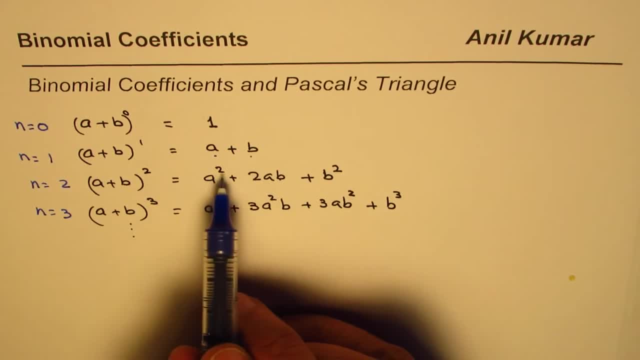 2. right degree of this term is 2. so what we notice here is that the degree of the terms is same as n, in this case a plus B, whole cube degree of each term is 3. when we say degree, so we are just saying the literal values, exponents when added up. 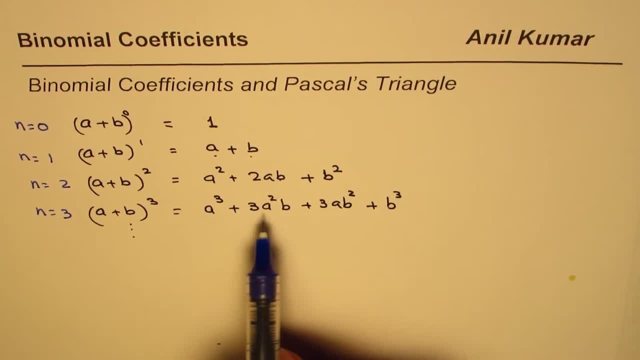 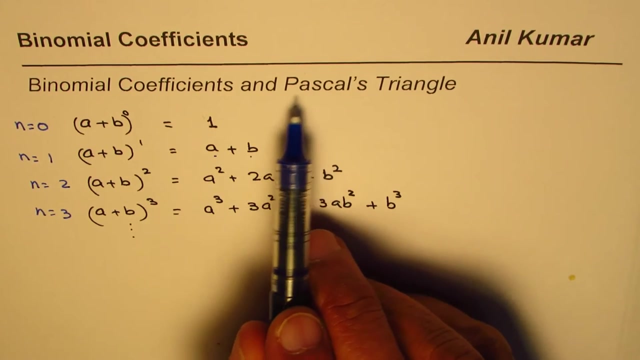 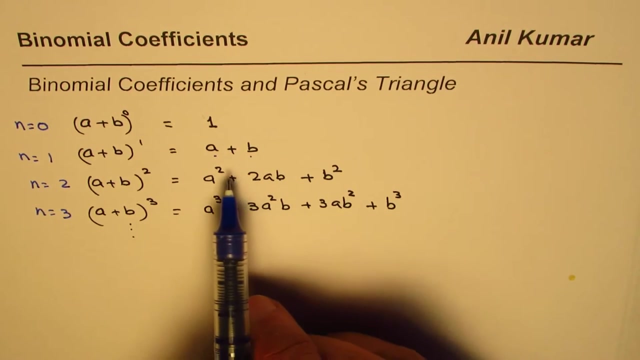 the. they give you the degree right of each term. so for each term, the degrees, what the value of n is. so there is also something which we learn from these expansion. now, the question we started with was finding a relation with Pascal's triangle. does it remind you something about Pascal's triangle? well, let's now. 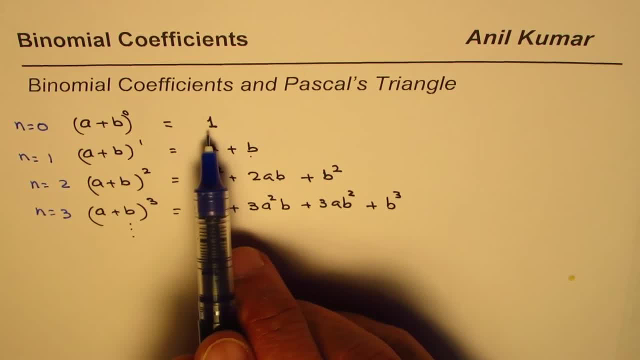 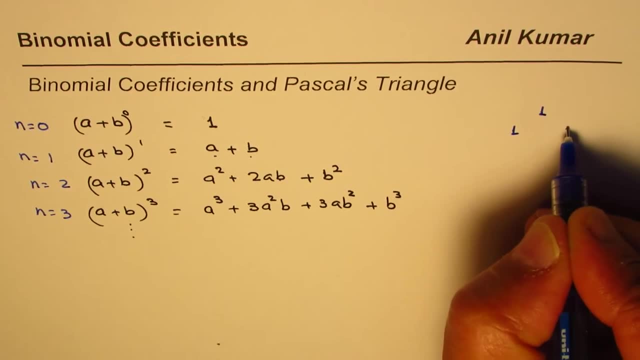 analyze the coefficients, right. so here we have coefficient 1. let me write down 1. in this case, coefficients are 1- 1. so I'm just writing coefficients 1 & 1, right? so let me just draw some arrows, just as we had in Pascal's triangle. right now here. 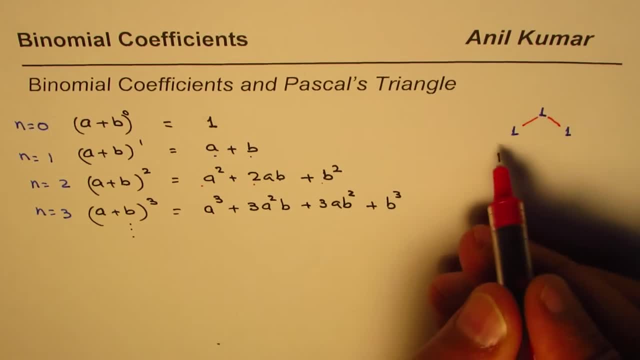 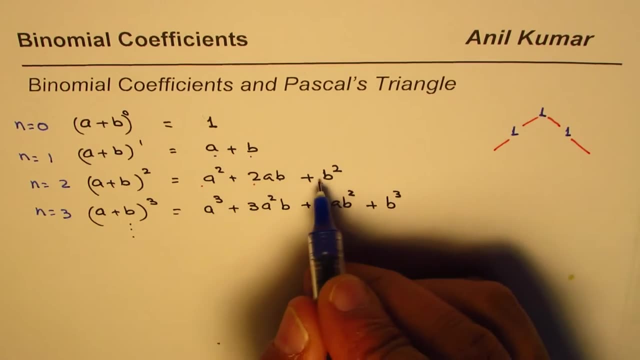 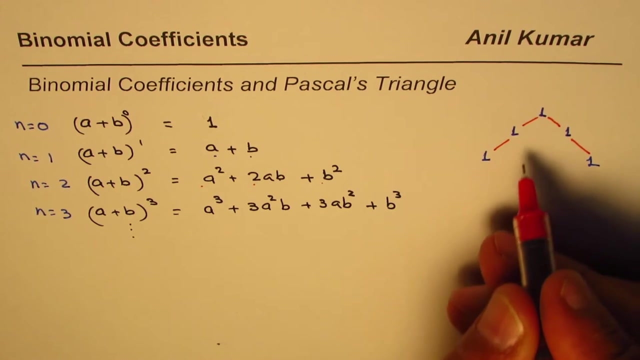 we have 3 coefficients. do you see that? so? so on the two sides, the coefficients are, as you can see, 1 right. 1 is coefficient of a square. 1 is coefficient of B square. the coefficient of the center term is 2, which you can get by combining: 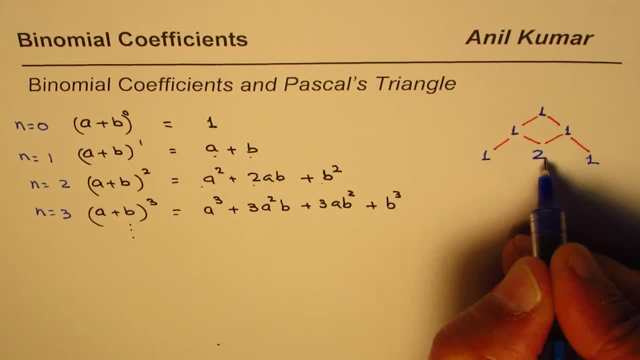 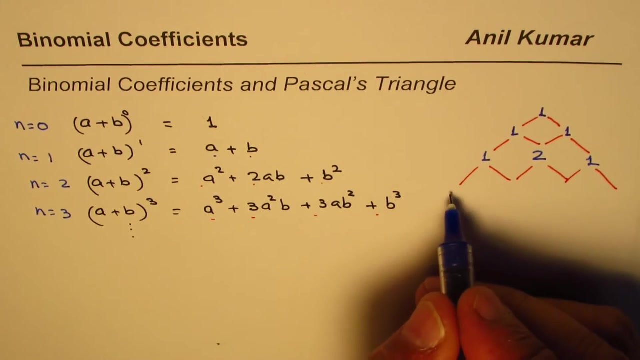 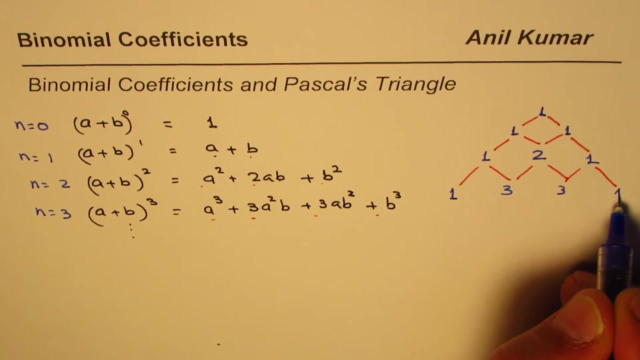 Combining 1 and 1.. Do you see that? So that is how you could get Pascal's triangle. Now, if I extend this pattern, as we did in Pascal's triangle, do we get the same coefficients as for Q? Well, this is 1,, okay, and then we have 3,, which is 1 plus 2, 3, again, which is 2 plus 1, and then 1.. So what we observe here is that the pattern being followed is similar to Pascal's triangle, right? 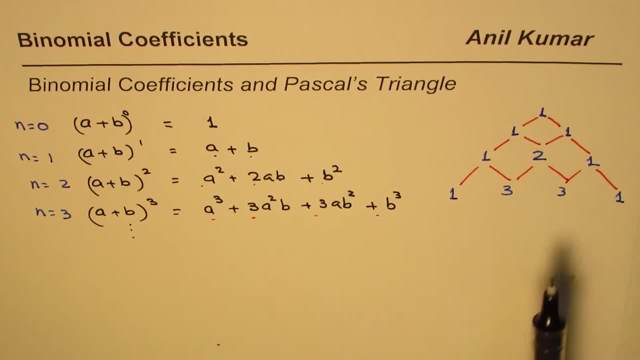 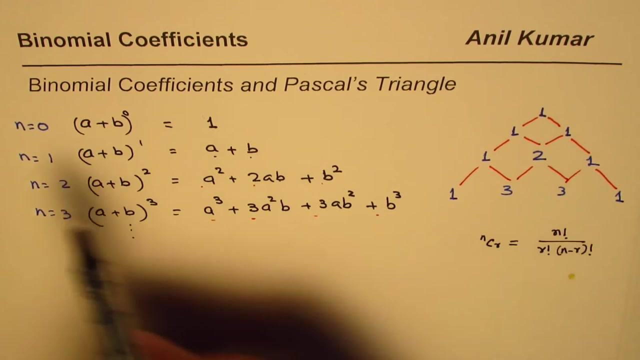 Now we will be referring to these coefficients as binomial coefficients, correct, Where The term- let me write here- nCr will be equal to n factorial over r factorial times, n minus r factorial. So that is the formula for the terms. Now, since we know, this is the term where n is 0, and we are calling this as 0th. 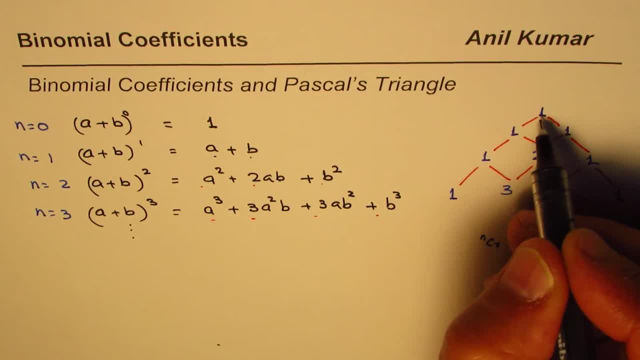 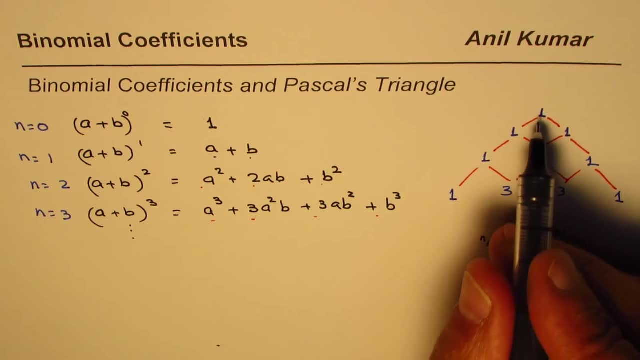 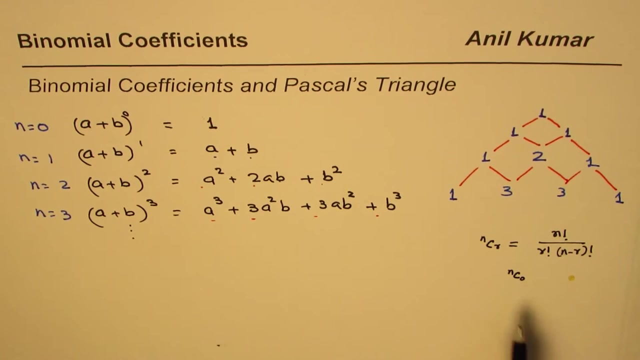 Column right. So in this case we can write this or replace this term by, let me write down here as nC0.. So here we are just calling about n. nCr was general. The first term here n is 0, right, So we will write this as 0C0, right. This term we are writing as 0C0. 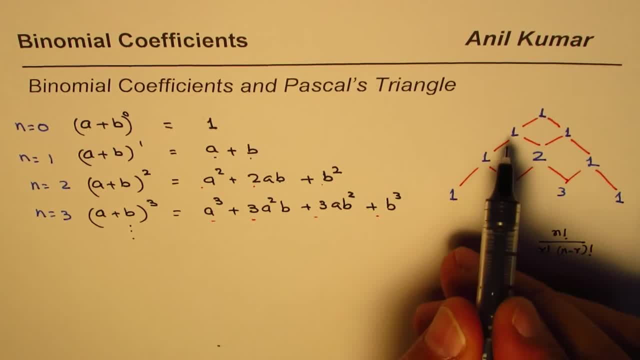 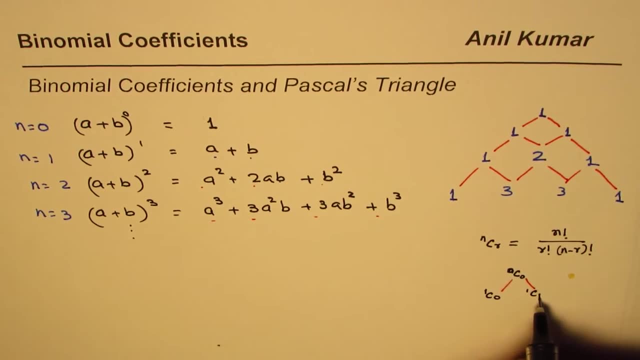 Then the next term Is where n value is 1.. So we have 1C0, and this one is 1C1,, correct. And then we have the. so this is row number 0,, row number 1, and then we have row number 2.. In row number 2, it is 2C0,, 2C1,, 2C2, correct. 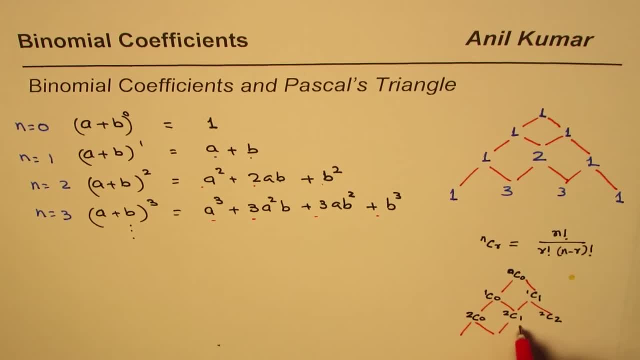 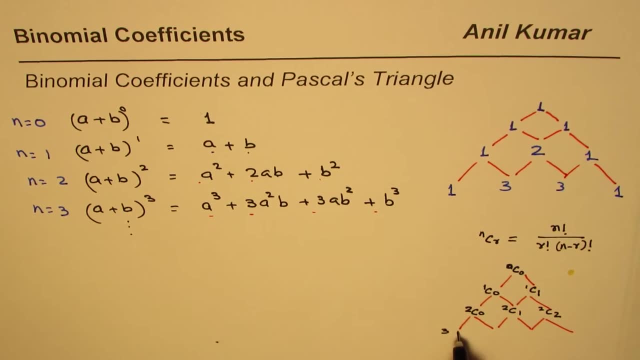 And in the third row, what do we get? In the third row, we get 3C0,, 3C2,, 3C1,, 3C2, and 3C3, correct. Now, if you calculate these binomial coefficients, you will get the same values. 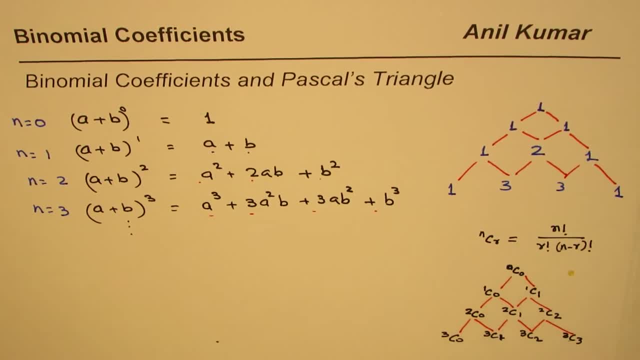 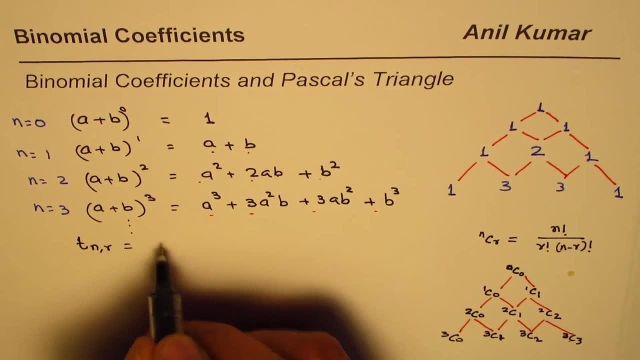 So what we see here, that in general, in general, from here we can say that T, nR is equals to. Sometimes we also write this as CnR. We sometimes write as, like this vector form, We also write this as nCr, as we have been writing correct. These are different ways of writing these binomial coefficients, but there is one-to-one correspondence between the Pascal's triangle and the binomial coefficients, correct? 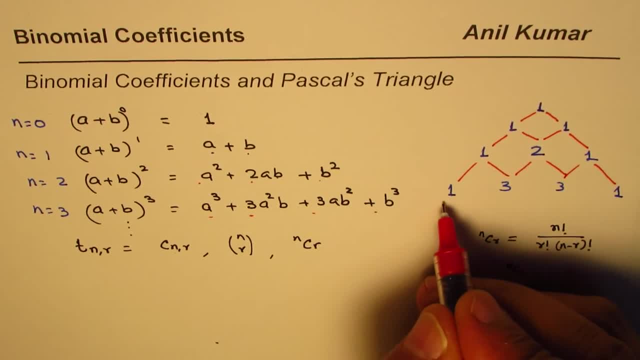 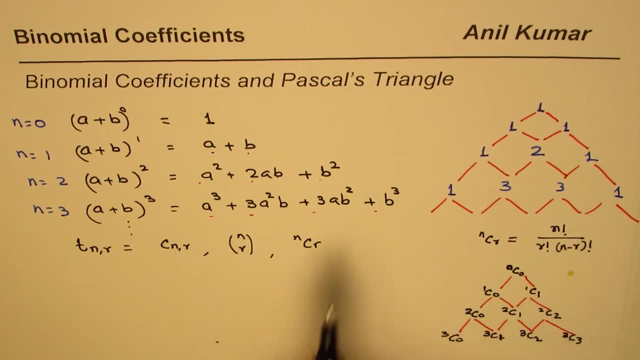 So using this you can actually also find the fourth power of binomial. that is, if you use this pattern, then you can write a plus b to the power of 4 as equal to. I will write in terms of these coefficients. It becomes kind of simpler. So we'll say 4C0a, right? 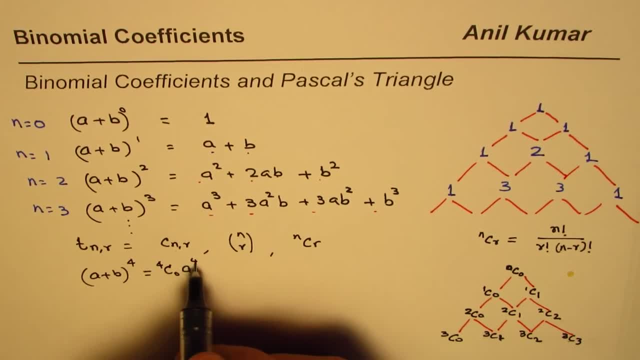 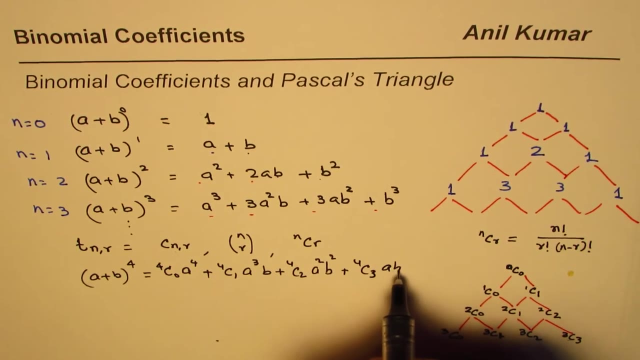 So a to the power of n, which is 4, plus 4C1aq, and the other term is b, then 4C2a2b2, plus 4C3abq plus 4C4. Now a power becomes 0, and b becomes 4.. So I'm not writing a to the power of 0. 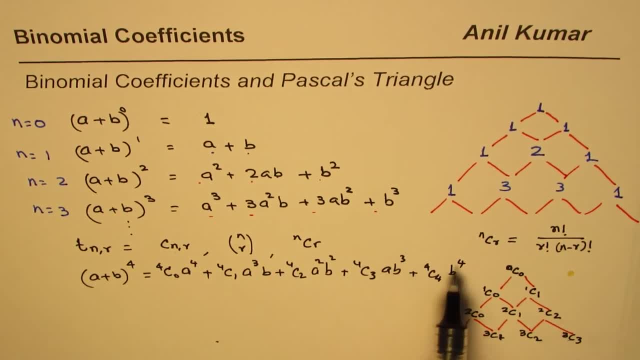 But the idea here is that this combination of exponents is always 4, right. Each coefficient is same as its position on the Pascal's triangle, correct Written in this form, which you can calculate right. So if you calculate these basically, it means if there are 4 items, choose 0. 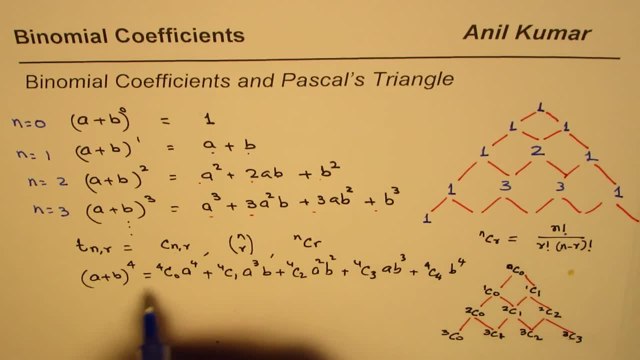 That is only one way. you can choose from 4 items. None of them right. So what we are trying to say here is: You have 4 items right, Choose 1 – I mean none right, None of them. 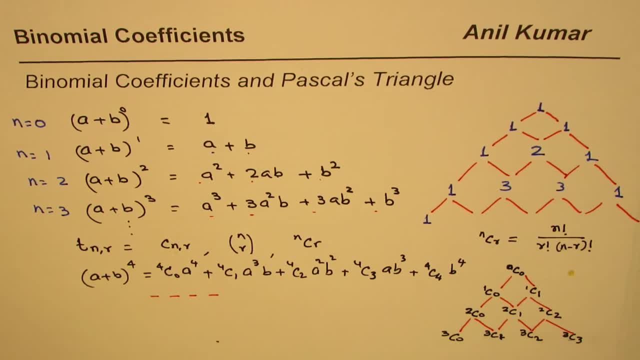 So when you choose none of them, there's only 1 way, one way. now you can see that if you have to select one of them, right. so you could select either this one, that one, this one or that one. that means these are four. 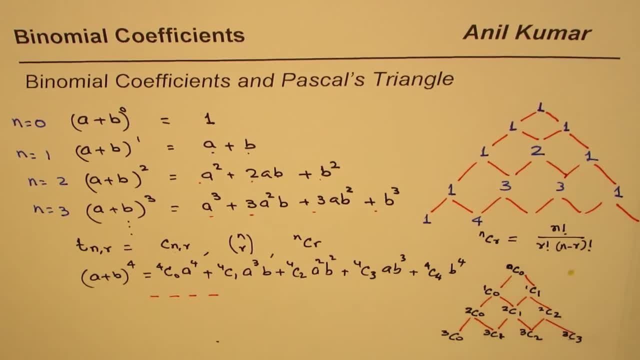 right. one plus three is also four, so you get that four. now, if you have to select two of them, then let me take up an example. let's say I will write on my name, Anil right. so if you select two of them with a, you could select n, I or L. so 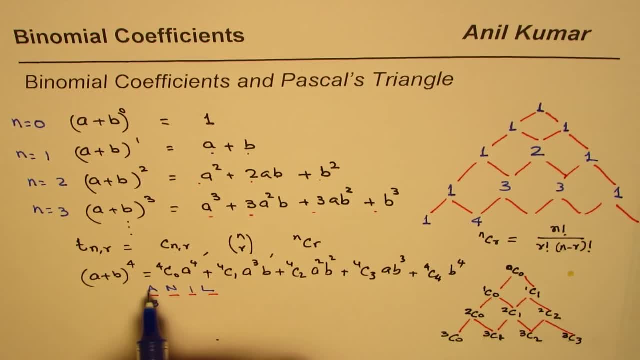 there are three ways, right with a, with n, we have already selected a, so you could select I or L. so there are two ways. with I, you could select L. so there is one more way. and when you add them up, you get the number 3 plus 2, 5 plus 1, 6. when 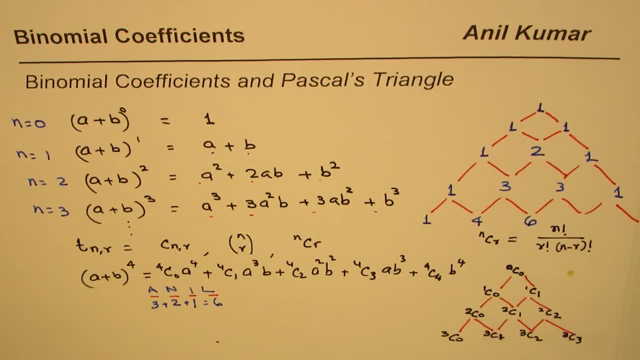 you add 3 and 3, you do get 6. do you see that? similarly, you can work out what happens when you select three at a time from four, right? so if you are selecting three at a time? so let me again take the same example, Anil. so so when you select three at a time, in that case you'll get four. 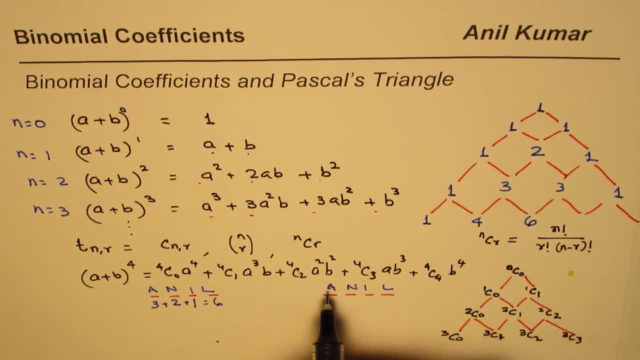 combinations. you can select Ani, right. so with a you could say Ni, or with a you could select Il or NL, correct? so these are three things you could select with a current and with n. what you can do is you could select a and i, which you have already selected, right. so when you select Ani, correct. so. 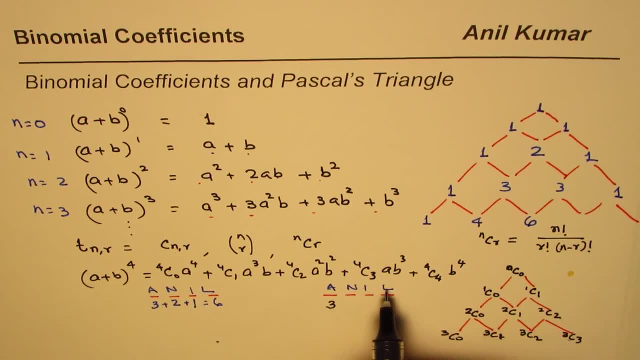 there's one more way. with n, you could select N i L. you get an idea right, so there is one more way. so once you do that, you have made all the selections, we three can be combined together, and so what you get here is four. Now the last one here is choose. 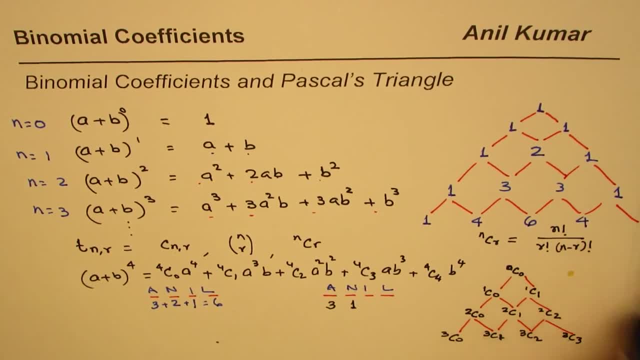 four out of four, So you have to choose all four. There is only one way to do it, So you fill that up. So what? you also see that these combinations, the coefficients, also follow the pattern that you add previous two to get the next one correct. So that is very important to understand. So what? 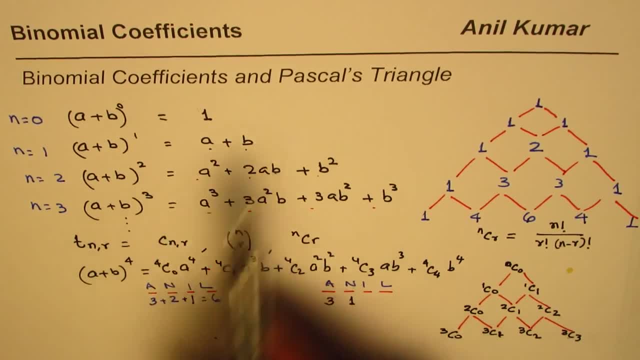 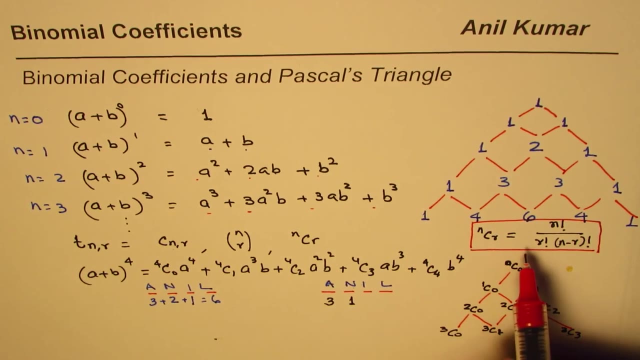 we have done here is we have linked binomial coefficients to Pascal's triangle with great significance, and that is now we have a formula. Do you see this formula here, NCR. So if I have to know what is the combination here, I don't have to start from the top: add and come to the stage.